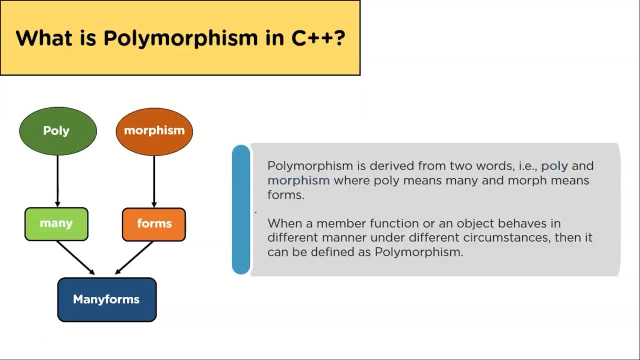 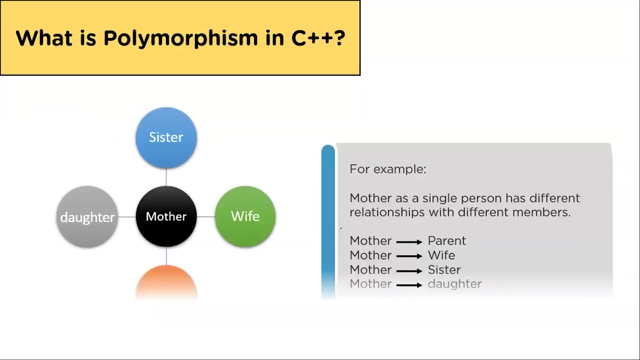 it means many forms. Polymorphism. in C++ can be defined as when the member function or the object behaves differently in different situations or circumstances. then it can be called as polymorphism. And polymorphism is defined as when the member has different relationships with different. 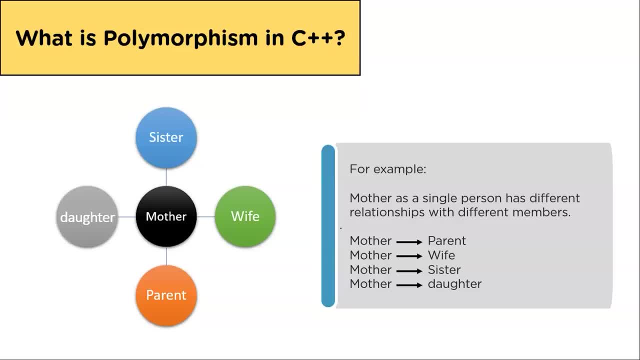 family member inside the house. For example, she is a parent to her child, she is a wife to her husband, she is a sister to her brother and she is also a daughter to her parents. So we can say a mother as a single entity has different behavior among different members. 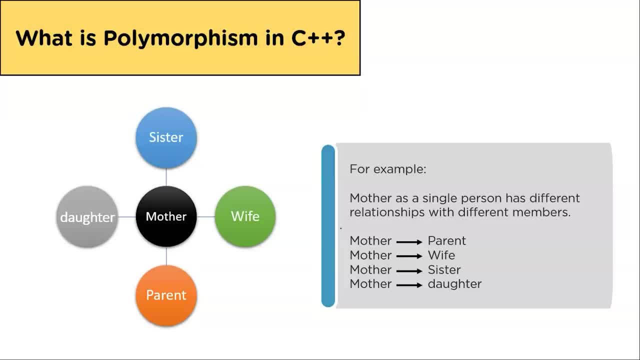 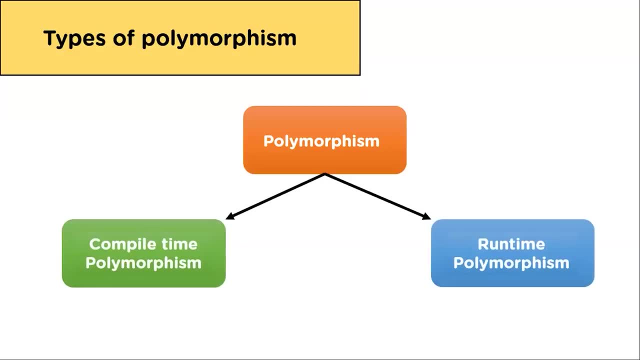 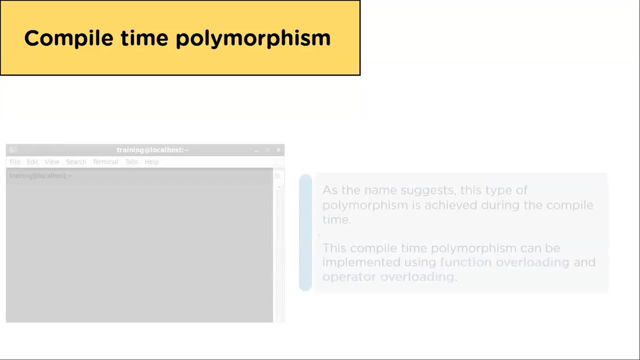 And same goes for polymorphism, where functions behave differently in different situations. types of polymorphism: There are two types of polymorphism in C++, that is, compile time polymorphism and runtime polymorphism. So let's start with compile time polymorphism. 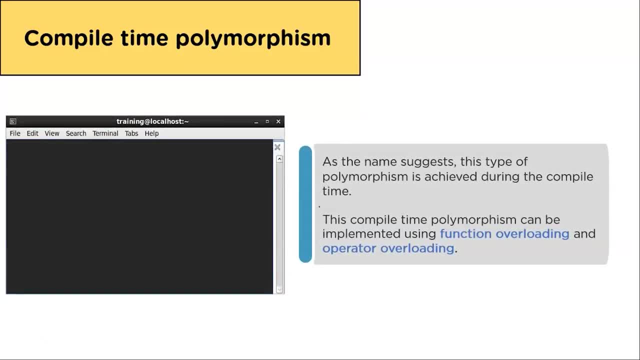 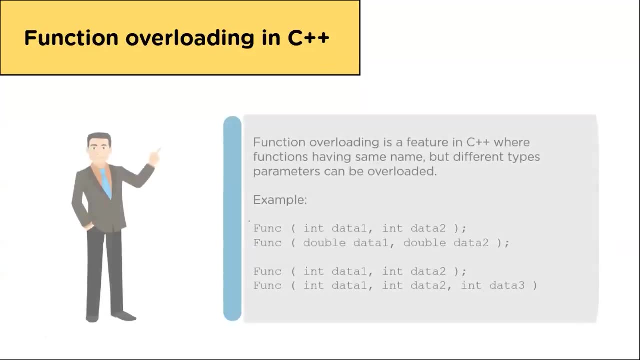 As the name suggests, this type of polymorphism occurs during the compile time and it is achieved by overloading the function or overloading the operator, that is, by function overloading or operator overloading. So what is this function overloading, Function overloading? 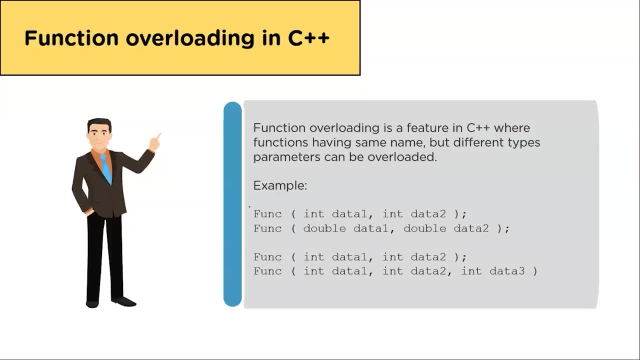 is a feature in C++ where the functions having the same name but different in terms of parameters or type of parameters can be overloaded. For example, as we can see two functions with same name func differ in the type of arguments. One data type is double another data type. 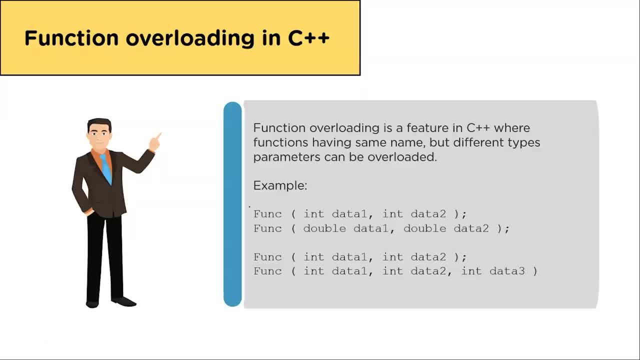 is integer. So when we make a call to the function, we will invoke the function. with arguments of type double, It will invoke the suitable function and the same goes for the other one. In example two there is a difference in number of parameters among functions. So while calling the function, if we pass two 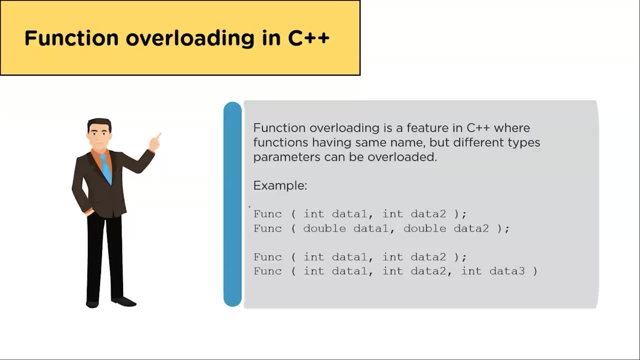 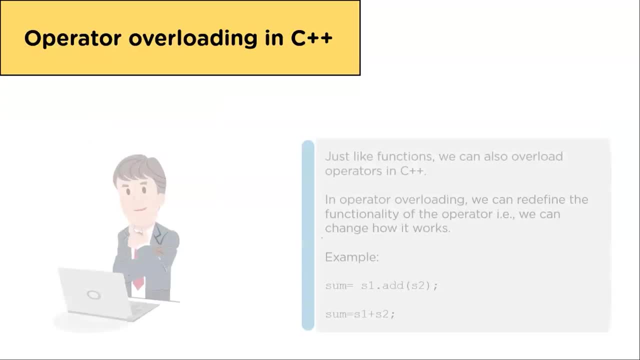 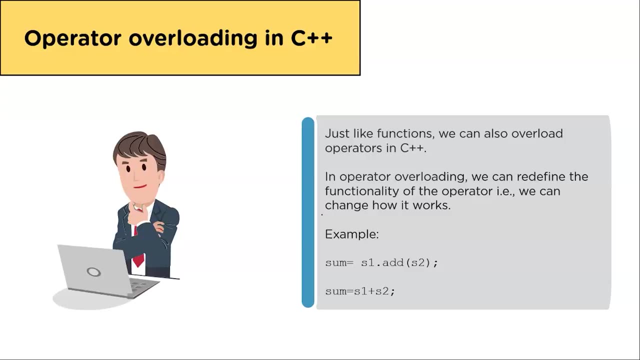 arguments, it will invoke the first function, and if we will pass three arguments, then it will invoke the second function. Then next is operator overloading. Like function functions, operators can also be overloaded. In operator overloading we can redefine the: 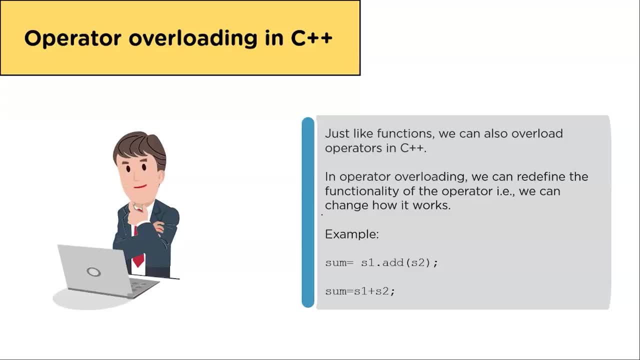 functionality of the operator. It helps us in redefining the already existing operator. For example, instead of writing sum equals s1, dot add s2,, we can easily write sum equals s1 plus s2.. That is, we can redefine the plus operator and use it to add the numbers in. 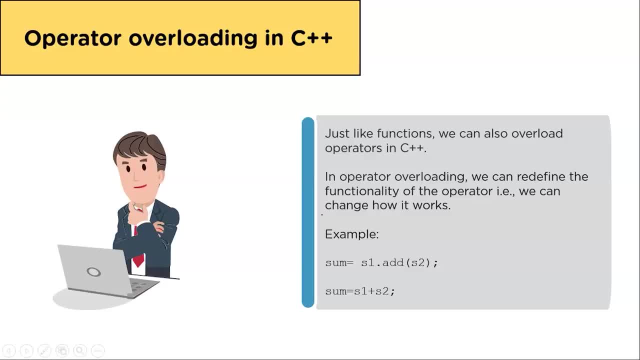 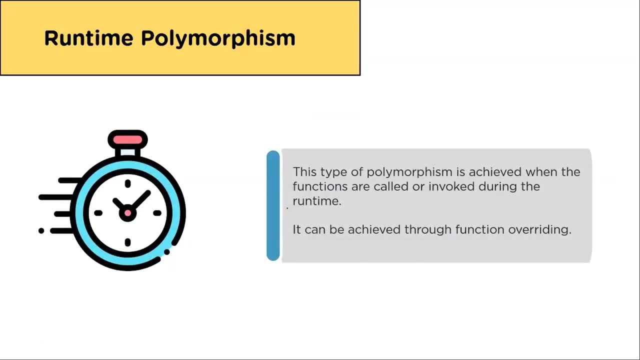 the operator function, And we will discuss the syntax of operator overloading in the examples. Now coming to runtime polymorphism: In this type of polymorphism the functions are invoked during the execution of program, ie during runtime. This runtime polymorphism can be: 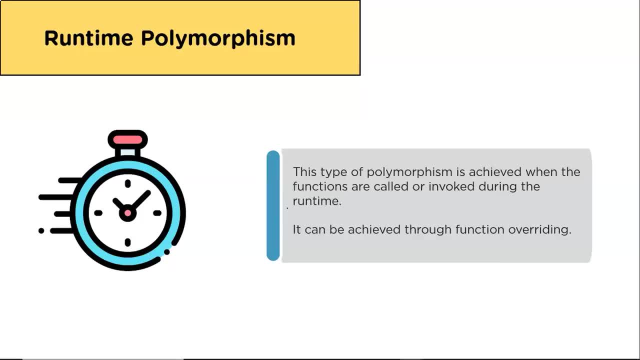 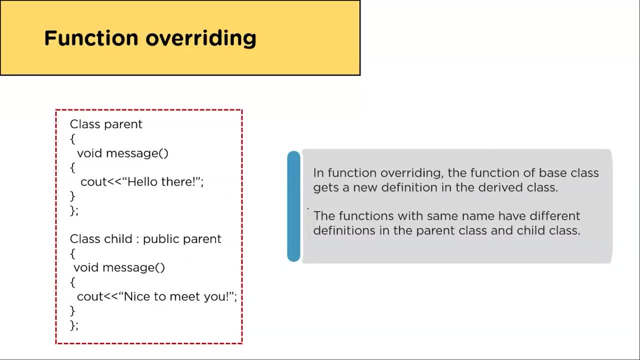 achieved through function overriding. So let's understand this function overriding. In Function Overriding we use the functions that are used to perform the operation of The function of the base class gets a new definition in the derived class. In this more than one function has the same name and same type of parameters. 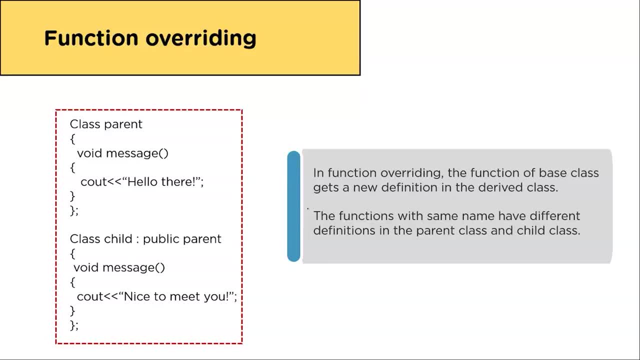 The only difference is in the definition of both the functions, That is, functions have different definitions in the parent class and the child class. As you can see in the example, void message function has a different definition in the parent class and in the child class. 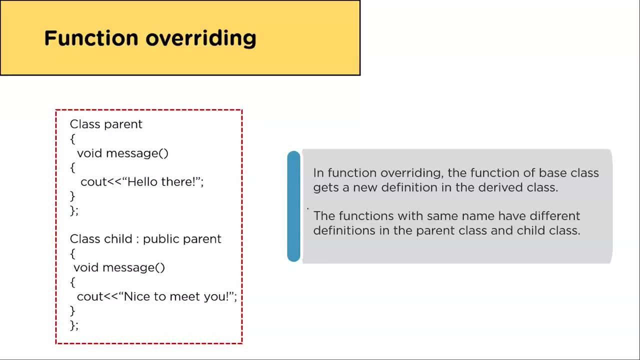 Both have the same name, but in parent class it is printing hello there and in child class it is printing nice to meet you. By using the object of the base class or derived class, we can invoke the suitable function. So let's move on to our next topic, that is, virtual function. 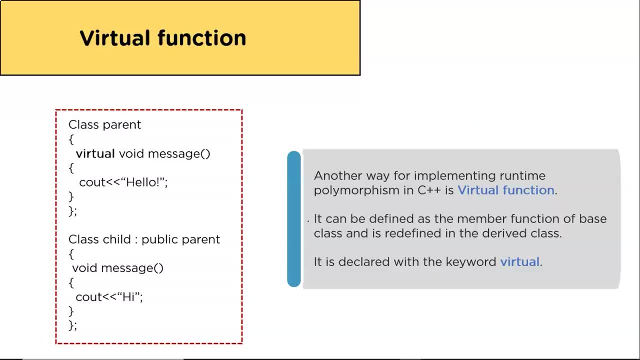 Virtual function is also used to achieve runtime polymorphism. It is a function that is defined in the base class And then is redefined in the derived class. The function is defined using the word virtual in the base class And the name of the function is same as that of the derived class, having different definitions as shown. 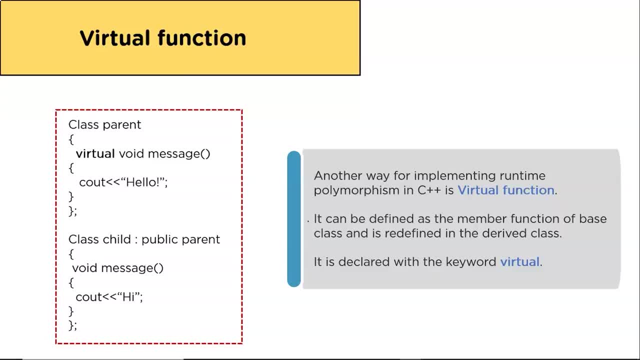 It tells the compiler to perform the late binding on the function in derived class. The function call is resolved at runtime and in late binding, And the compiler determines the object type at runtime. With the help of virtual function, We can invoke the derived version of the function in the derived class. 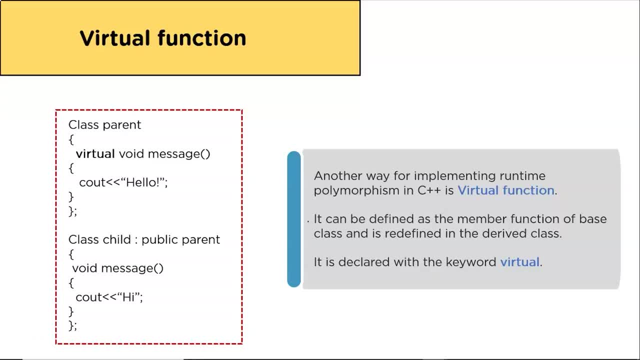 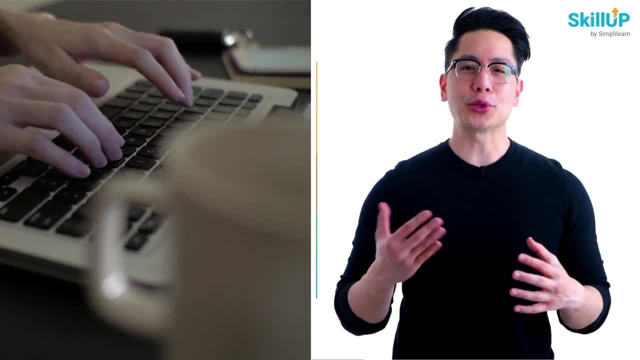 So as we have covered the theoretical aspect of C++ polymorphism, So let's go ahead and cover the practical aspect of this topic in our code editor, that is, VS Code. If getting your learning started is half the battle, What if you could do that for free? 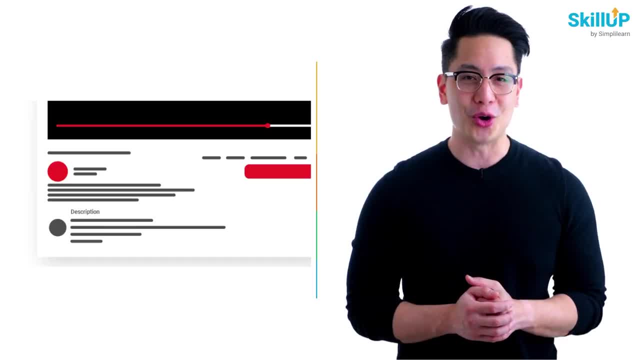 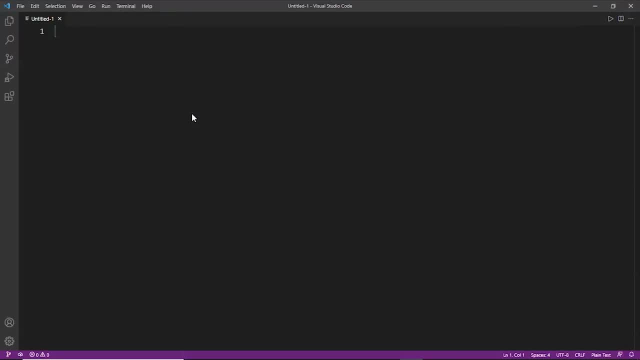 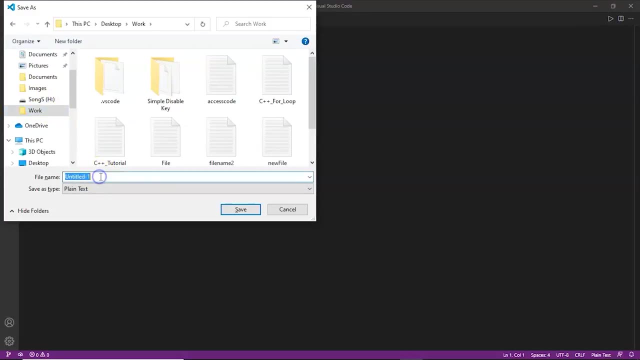 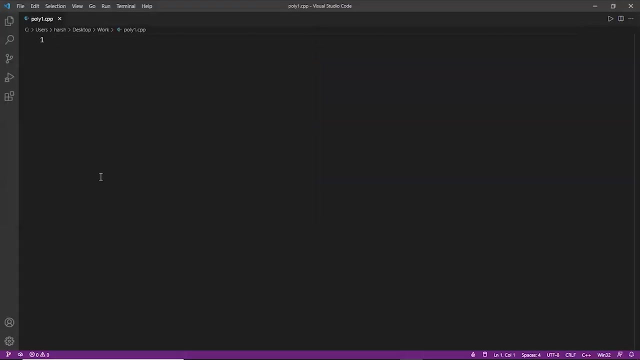 Visit SkillUp by SimplyLearn. Click on the link in the description to know more. So here we will make a new file And let's name it as poly1.cpp. Alright, poly1.cpp, Let's save it. So here we will do an example of function overloading, which is used to achieve compile time polymorphism. 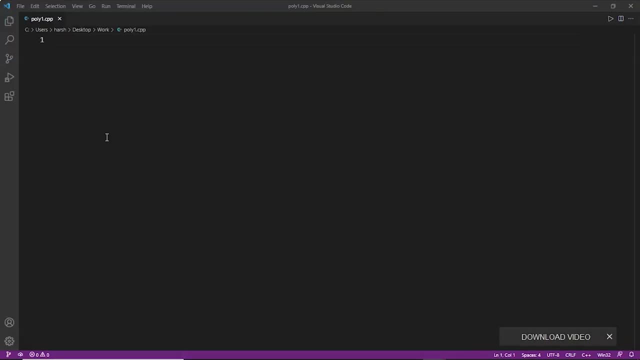 And we know, function overloading is a feature in C++, in which two functions have same name But differ in terms of parameters or number of parameters. So the type of parameters can be overloaded. So let's start. First of all, we will write the header file. 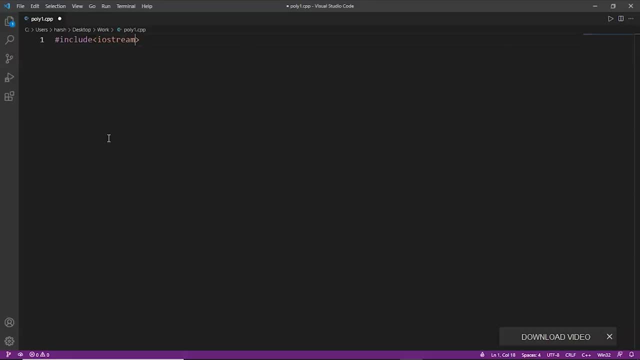 hash. include iostream, Now using namespace standard. Alright, So now we will create a class king and inside that class we will do the overloading. So the class name is king And inside the class. First of all, let's make public scope. 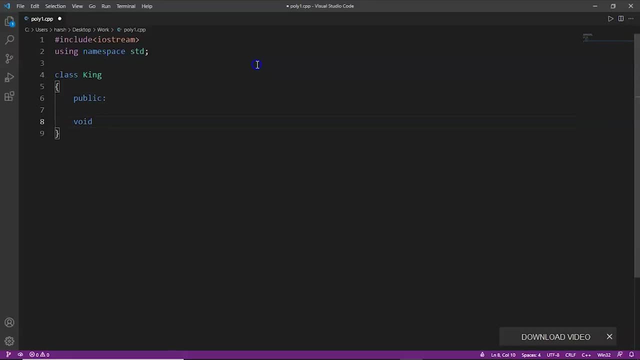 Now we will create a function. Return type is void And the name of the function would be pro Inside this function. let's say we are passing two arguments int. a and b. Alright, Now we will print both of these arguments or variables inside this function. 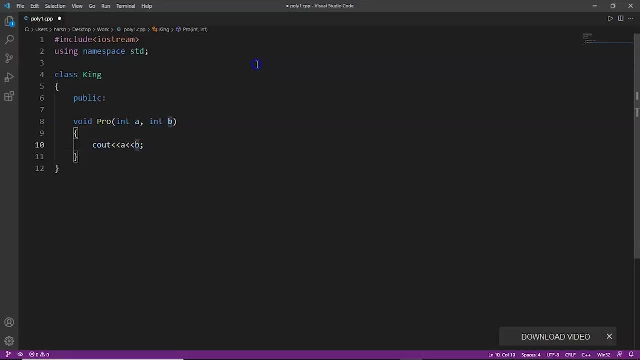 Alright, And we will use endl in the end. Okay, After that, we will create another function And the name of the function is same. that is pro And, but in this case we will make the arguments like int a, int b, int c, int d and int e. 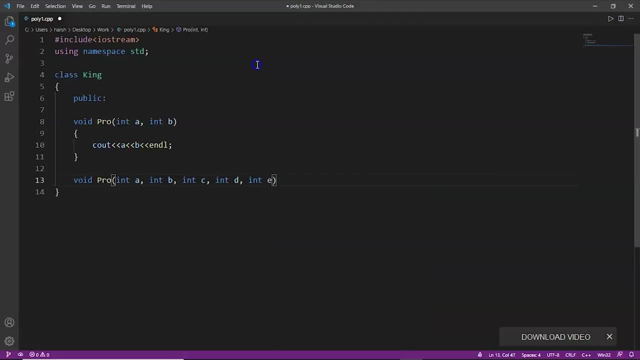 So there are five arguments in this function. Second function pro. As we know that the name of the function is same, And now, inside this function, we will simply add all of these, So a plus b plus c, plus d plus e. Alright, 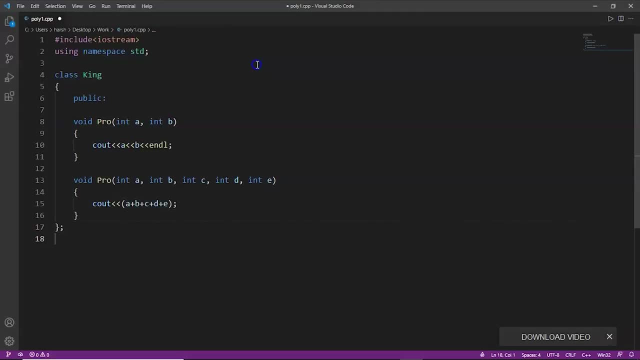 Once we are done with this, We will use semicolon in the end of the class. Alright, Now we will start with the main function. Inside the main function, Alright, Inside the main function, We will create the object of king class. 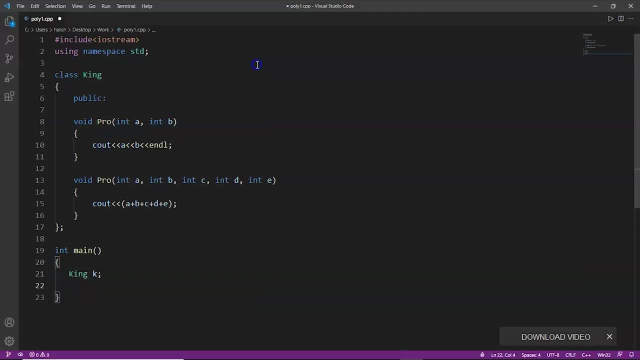 King, and the object would be k. With the help of this object, k. We will call these functions. As we know, the name of the functions are same. The only difference is in the number of arguments, So I will call the pro function. 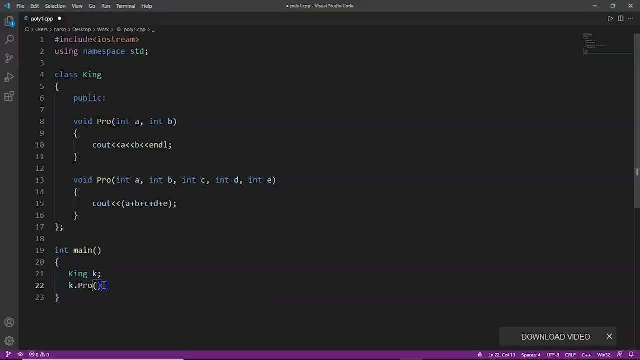 Which accepts only two arguments. So the first pro function will be invoked. So I will pass 10 and 20.. So these two arguments will be passed over here, Alright. Similarly, Now we will call the pro function again, But now we will pass five arguments. 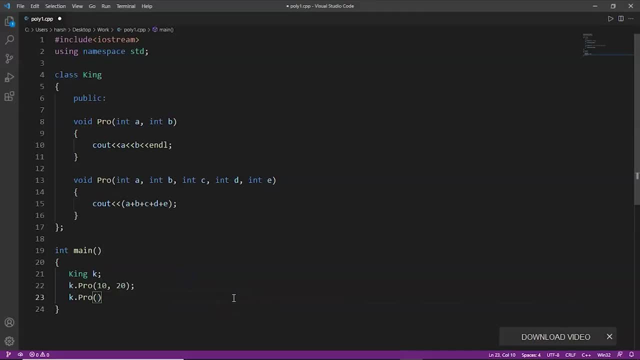 So that the second pro function would be invoked. So let's say I am passing 12,, 23,, 20 and 60 to 6.. These are some random numbers. Alright, Now return zero in the end. Now let's try to run this. 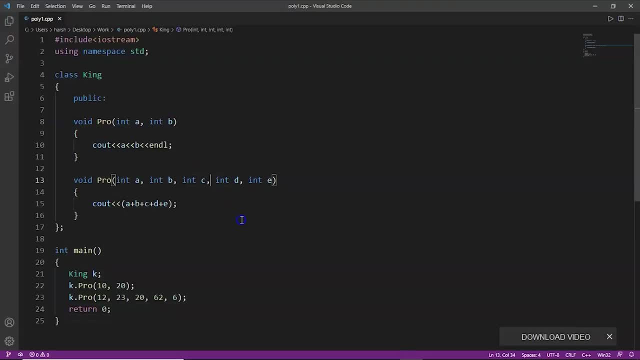 I think we are done with this. First of all, let's save it, And now let's try to run this. So this is our output: 10, 20.. Let's make it. Let's multiply both of them. It will look good. 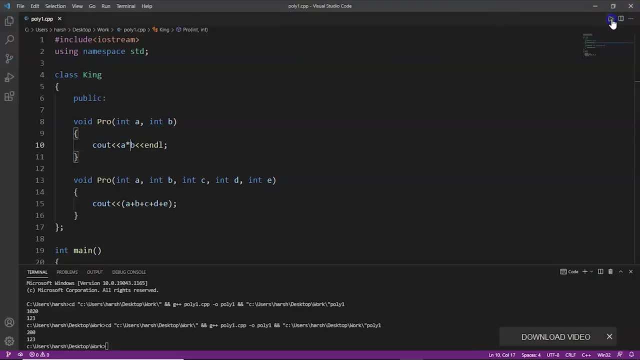 Let's save it. Let's run it again, As you can see: 200 and 123.. So this is our output: 10 into 20 would become 200. And if we add all of these, we will get 123.. So this is our correct output. 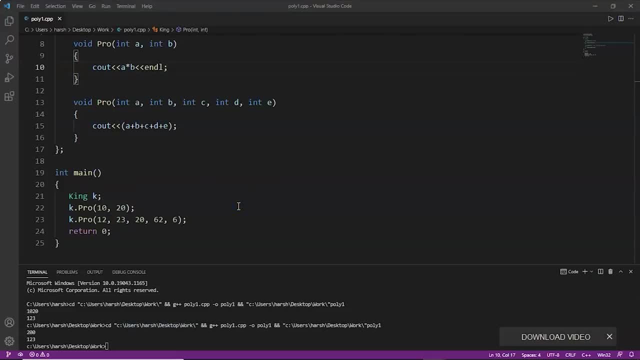 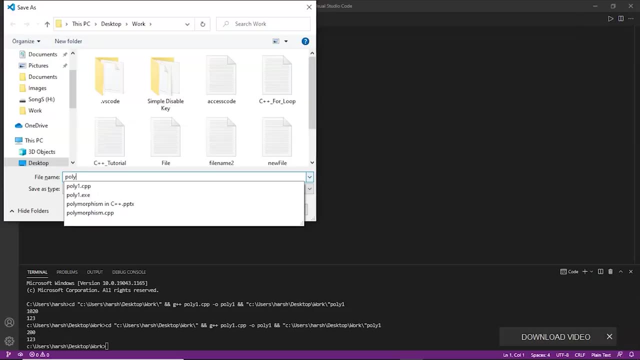 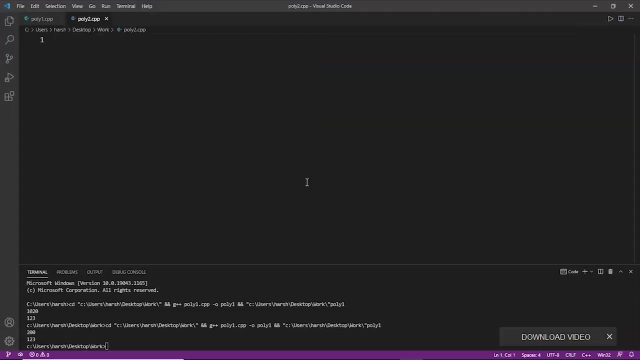 So this was the example of function overloading, And let's start with another example. So now let's create a new file And name this file as poly2.cpp. Alright, We have saved it. Now, here we will do an example of operator overloading. 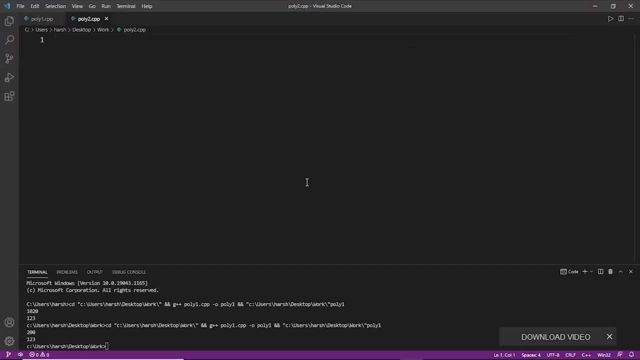 As we know that in operator overloading we give definition to already existing operators, Or we can say we can redefine the functionality of already existing operators. So let's start. First of all, we will include the header files, as we have done previously. Hash include iostrain. 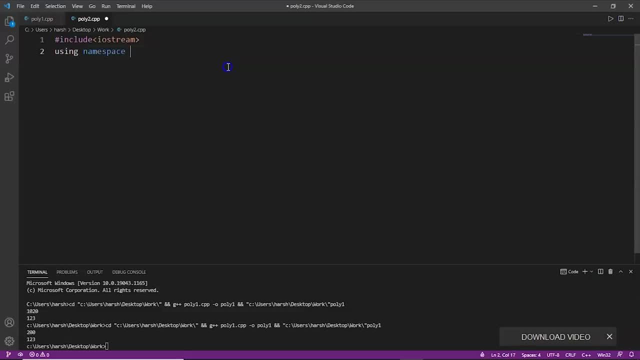 Then the namespace standard. So first of all we will start with the main function And inside the main function we will write the name of the class that we will create And the object. Let's say the name of the object is 01.. 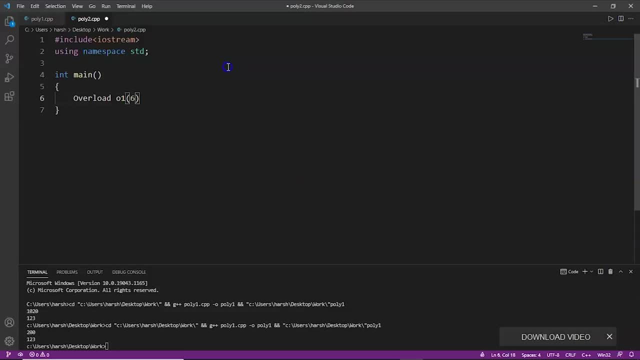 And we will pass the arguments to the constructor. Let's say the argument is 6 and 8.. Alright, Then I think we can write return 0. And we will do the rest afterwards. First of all, we will create the class. 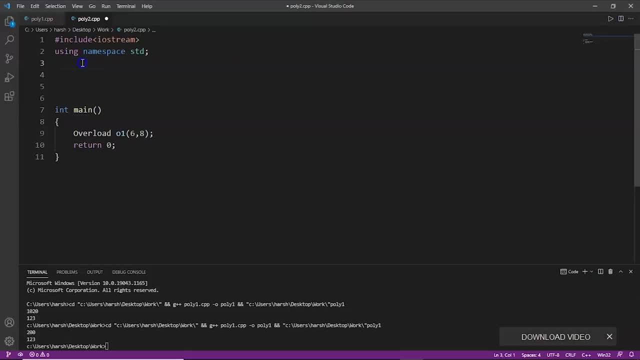 So, as we know that the name of the class is overload, So let's create it, Class overload. And inside this class, Inside the private scope, We will start with the variables. Let's say the first variable is n1.. And let's declare another variable, n2.. 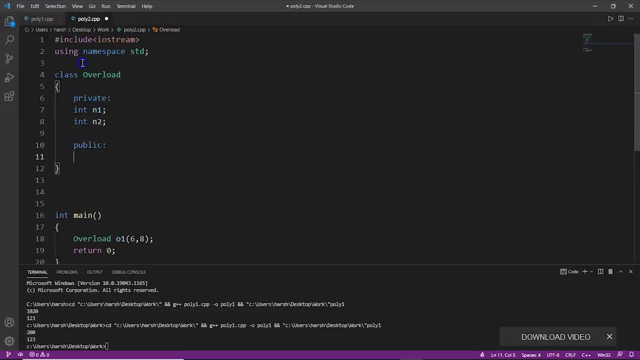 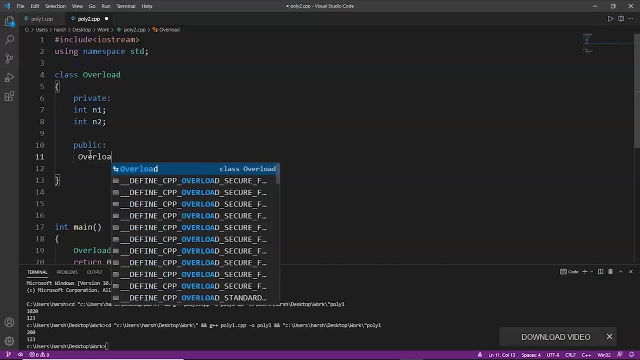 Then we will create the public scope. Inside this we will create the parameterized constructor, So it is of same name as that of the class that is overload. And now, as the constructor is parameterized, So int num1 and num2 are the parameters. 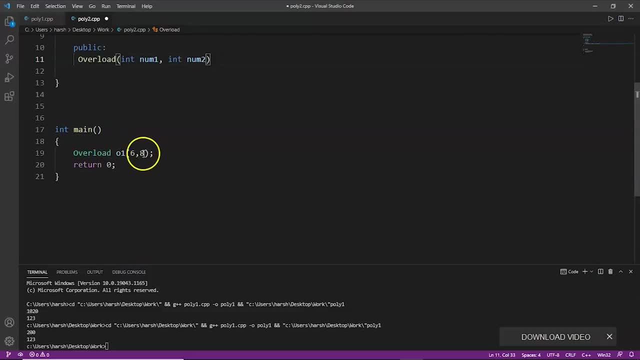 So when we will create this object 01.. And we will pass these arguments, So it will go here And alright, Inside this, in the definition of this constructor We will create, We will declare the variable rest And we will assign num to n1.. 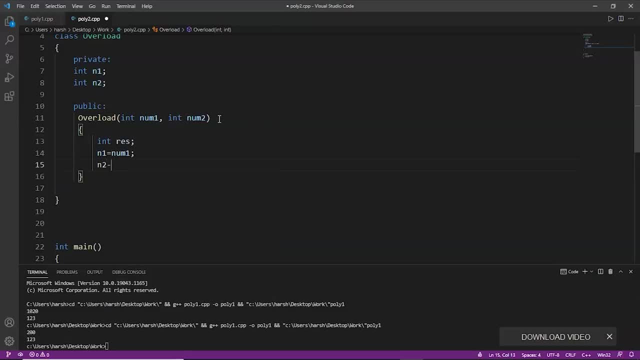 We will assign num2 to n2.. And let's say we will do the subtraction: Alright, n1 minus n2.. Alright, Now we will display the result, that is, rest, So res, And then the variable rest. After that we will use zendel. 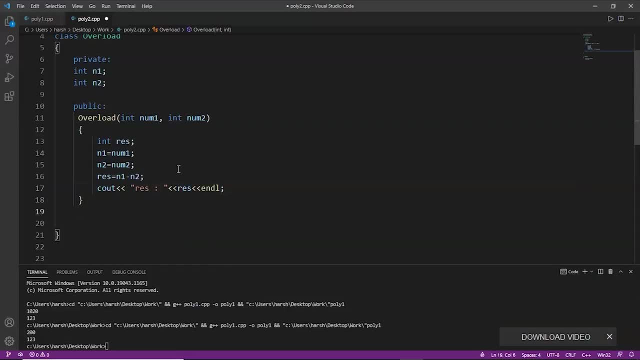 Alright. So once we are done with this parameterized constructor, Then we will create a operator function. So void is the return type. Then we will write operator keyword. This is the syntax of operator function. Then, after writing the keyword, We will write the symbol. 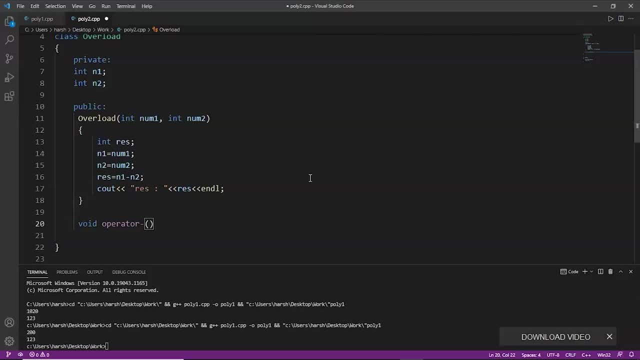 Let's say: minus is the symbol, Then the arguments. If there are any arguments, Then we can put those Then inside the function, that is in the definition. We can perform whatever the functionality we want to perform. So let's say in this case: 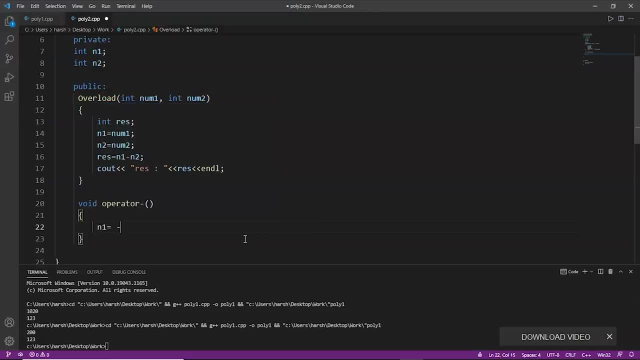 We will just make the numbers negative. So we will do that. Alright, Now we will do the calling part of this. We will simply use the symbol and the operator, And this is how we will call the operator function. This is very simple. 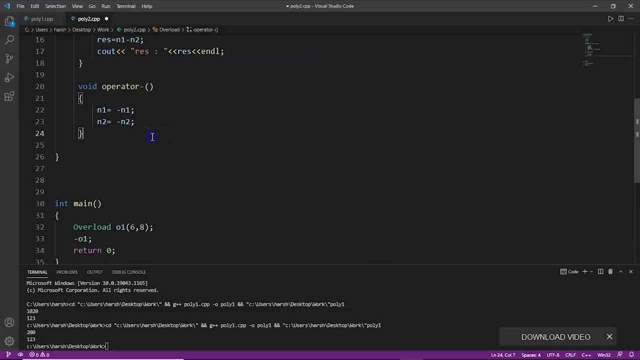 And after that we have to display the digits as well As we have made them negative in this part. So we will create a function display And inside this function We will display those digits or numbers. So we will write n1.. Alright, 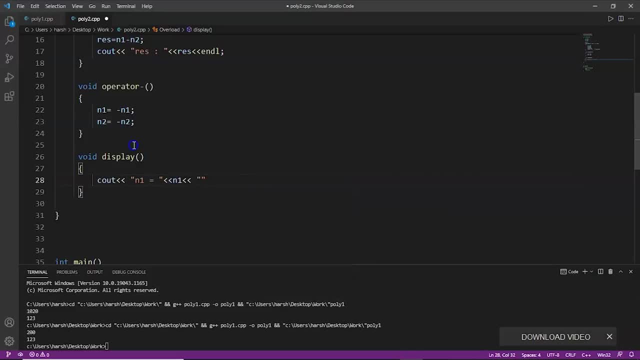 After this, we will write: We will do same for n2.. So we will write n2.. And n2.. Then there is ndel in the end. Alright, So here we are displaying this. So once we are done with this, 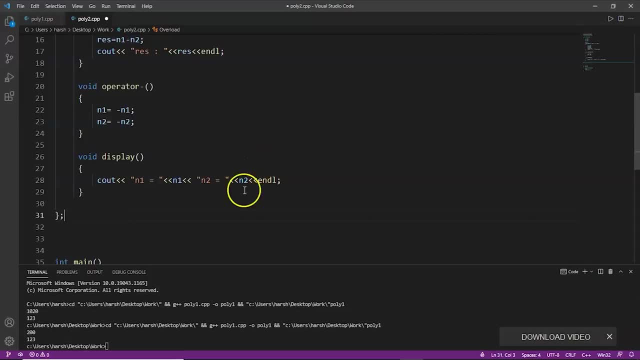 The class is finished, So we can use the semicolon in the end. And we have to call this void function as well, So we will write o1.display. Alright, We are done. Let's see whether it works or not. Let's save it. 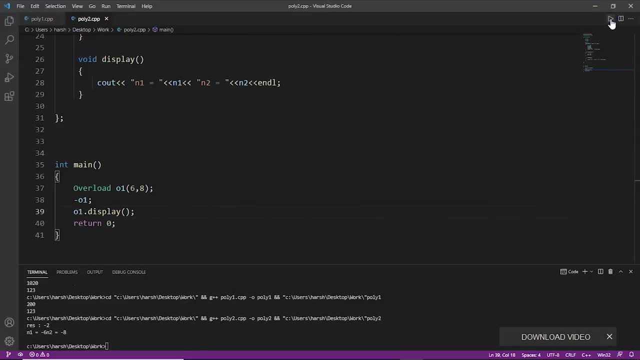 And check it So, as we can see, the result is minus 2.. That is, 6 minus 8 equals minus 2. That is correct. And n1 is minus 6. And n2 is minus 8. Because we have made them negative. 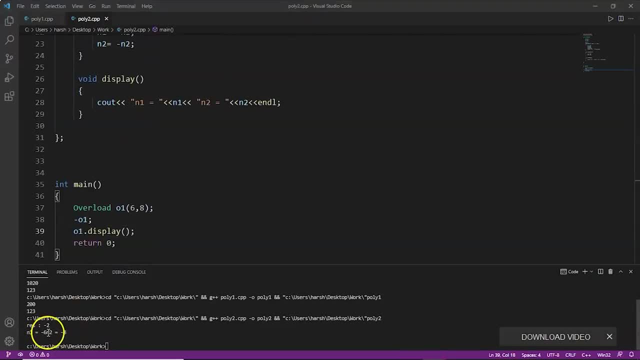 Inside this operator function. We forgot to add some space in n2 and n1.. That is why it is looking like this, But the answer is correct And this is how we can do the operator overloading. In this part we have used the return type. 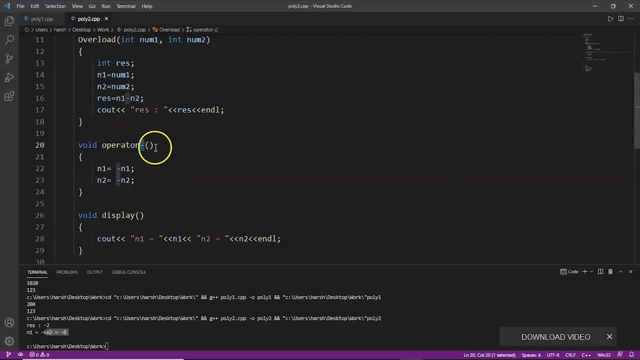 Then the operator keyword, Then the symbol, And if there are any arguments, Then we can pass those arguments, And if there are not, We can put it like this: So this is our example of operator overloading. Let's do another example. 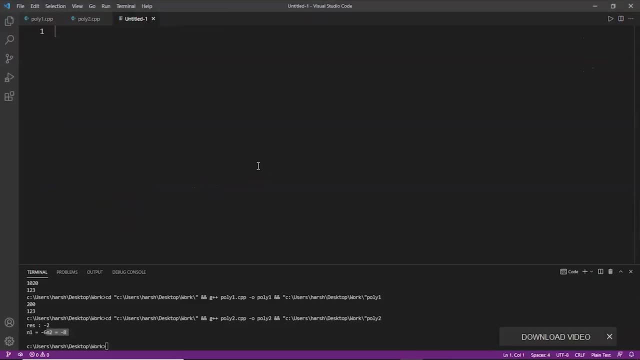 So now we will do an example of function overriding. So let's name this poly3.cpp. So in function overriding the function of base class gets a new definition in the child class, And when we call the function of the child class using the object of child class. 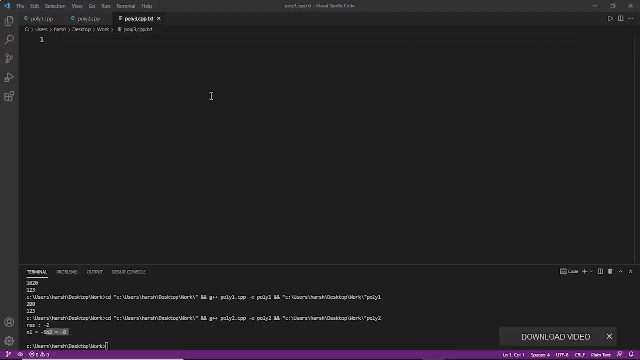 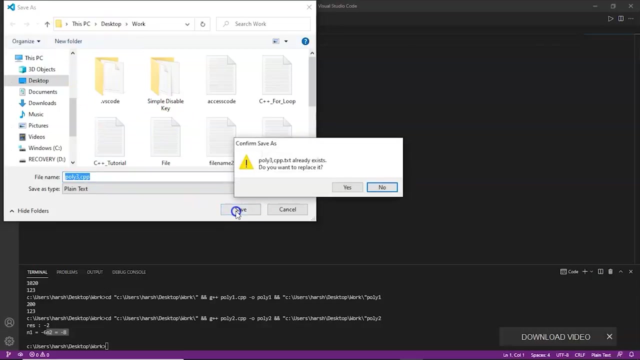 Then the function of base class gets overridden. So now let's do the example of this function overriding. I think we have named it wrong: poly3.cpp. Alright, Let's name it 4.. poly4.cpp. Alright, now let's save it. 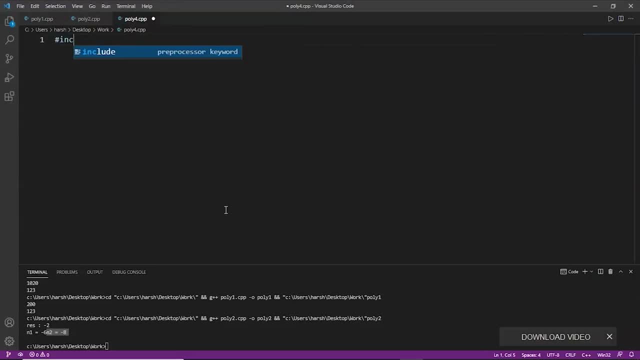 Now include the header files using namespace standard. Now we will start with the class parent. So this is the base class And we have named it parent. Inside the parent class we will create a function For that. we will create the public scope. 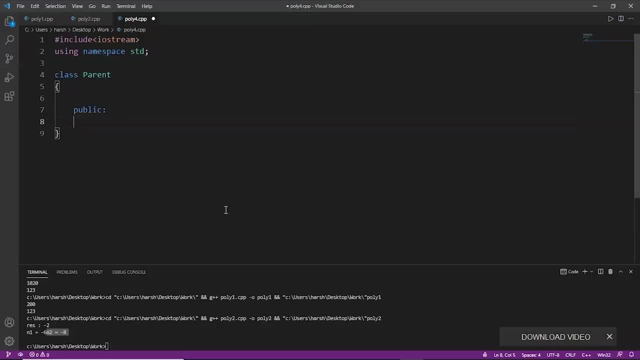 inside, Inside the public scope, we will create the function print And we will display the message. This is the function of parent class over base class whatsoever. Alright, So this is class parent And semicolon in the end of the class. Now we will create the child class. 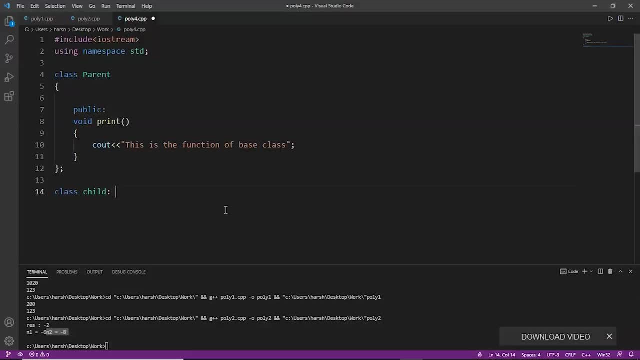 child derived from parent. class: Name of the class is parent. Similarly, we will do the public scope And create the function void print, void print. So it is same function as that of the above class And inside this function we will display. 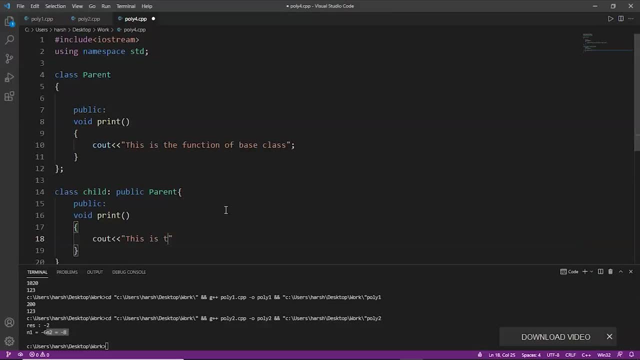 This is the function of child class, Derived class. let's say, Alright, Once we are done with this Semicolon in the end And semicolon in the end of the class as well, Then we can create a main function And inside the main function. 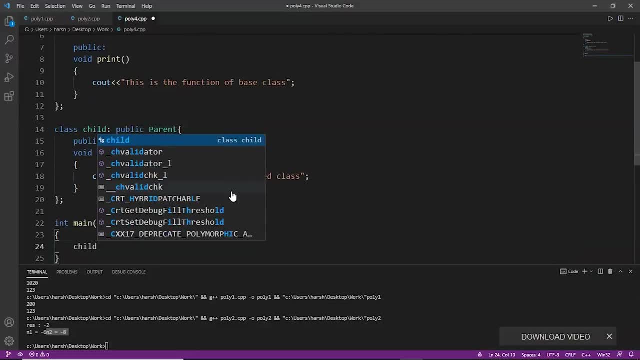 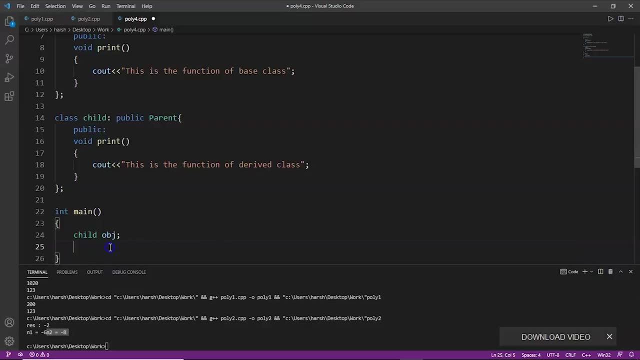 We will create the object of child class, child, obj. So, as we have created the object of child class or derived class, So with the help of this we will overwrite the function of the base class. So we will write objprint, Which is the name of the function. 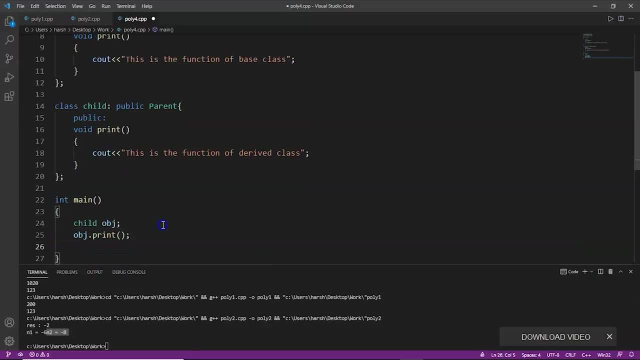 So as we have created the object of child class, So it will call the derived class or child class function And in the end let's say return 0.. Now save it And try to run this. This is the function of derived class. 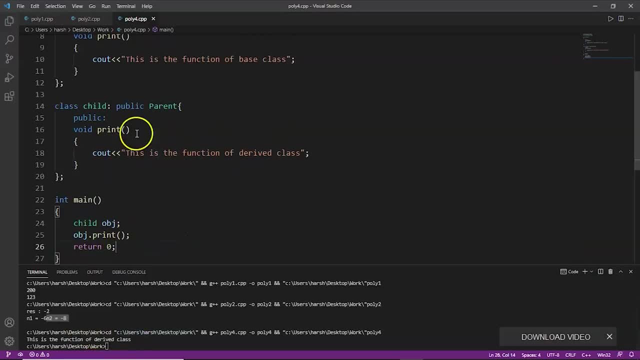 So, as we have expected, So it is calling the child class function, So this function of the parent class gets overwritten, As we have used the object of child class And call this function print, which is of same name, So this function, which is in the child class, gets to print. 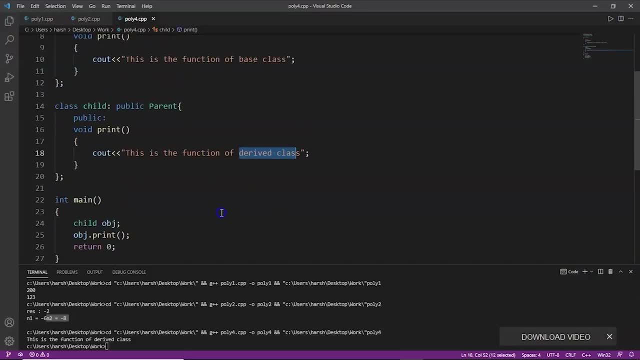 Derived class. So this is our output. So now let's do an example of virtual function in C++. Virtual functions are defined in the base class to ensure that The functions gets overwritten And when we use the base class pointer to hold the derived class object. 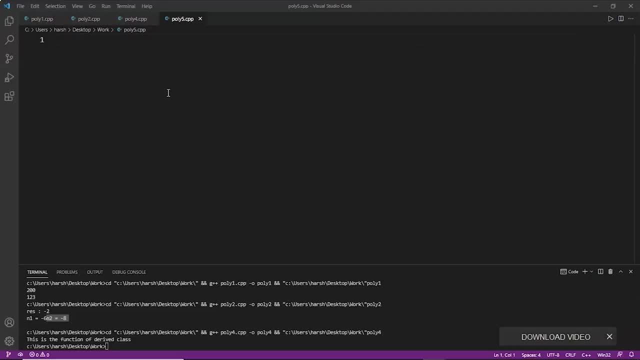 Or the child class object. The base class pointer will always call the base version of the function And not the derived version. So to solve this problem we use the virtual keyword in C++. So now let's start with it. First of all, we will write hash: include iostream. 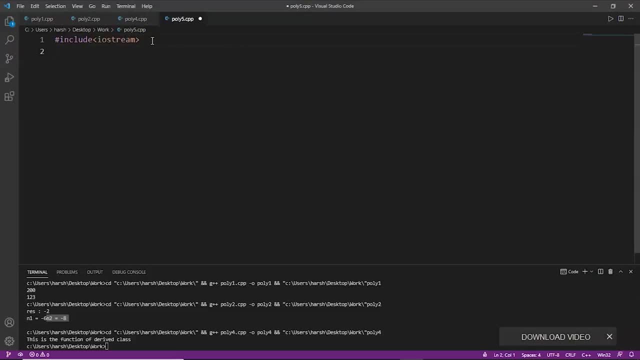 Now the namespace standard. Now we will create the base class, Class base, And then we will use the public scope. Inside the public scope, we will create the virtual function. Use the virtual return type, Then the name of the function That is print. 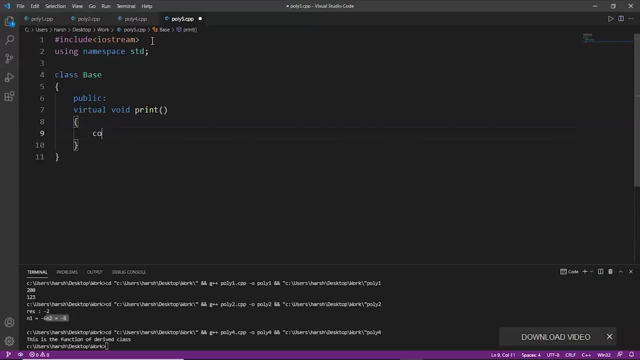 And we have created this virtual function inside the base class. Now we will print This is the function inside the base class, As we have done previously in the previous question. This function, This is the function of base class Here it could be right. 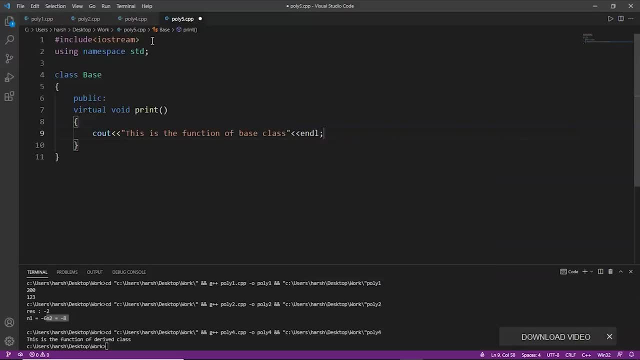 Alright, Once we are done with this, We will close the class by using semicolon. Now we will create the derived class And we will name it derived From the base class, whose name is base itself. Now, here we will use the public scope. 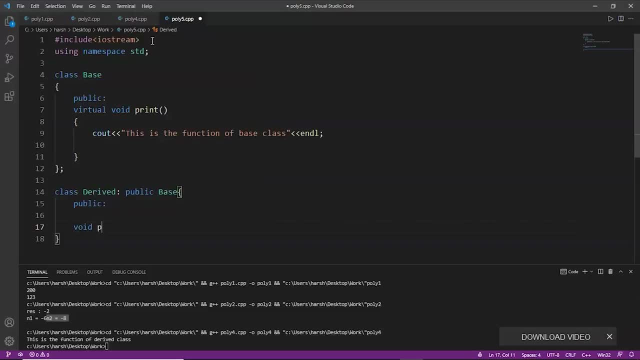 And we will create the function Of derived class Print function And we will print. This is the function of derived class. Alright, Now we will use the semicolon To end the class Now inside the int function: Int- main function. 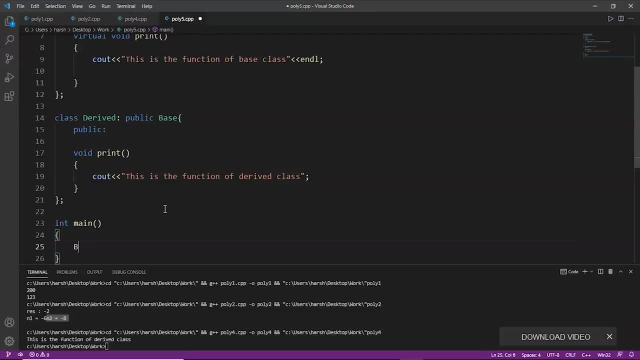 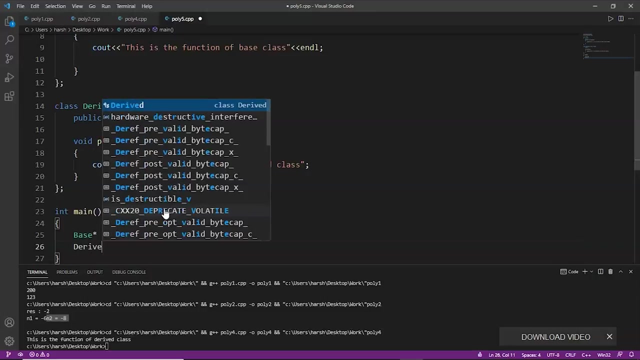 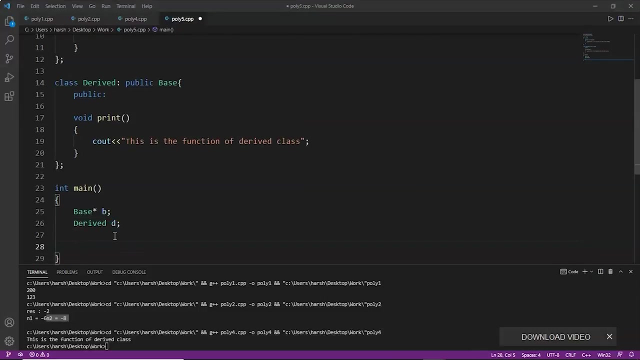 First of all, We will create the pointer of base class, Base D, reference operator B. So we have created the pointer of base class. Now we will create the object of derived class, Derived D. So now We will store the address of derived class object. 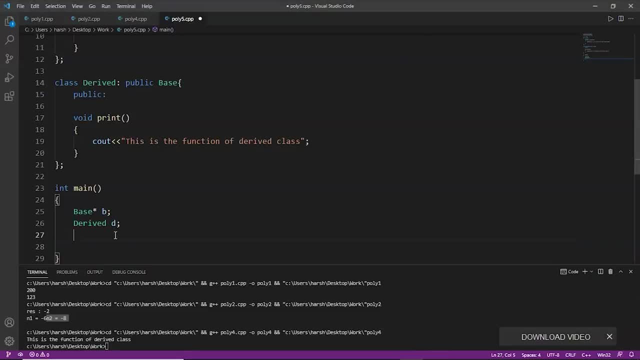 To the pointer of base class. So let's do that. B, Which is the pointer of base class, Address of operator, The object of derived class. So now we will call the print function Using the pointer of base class And it will print the derived class function. 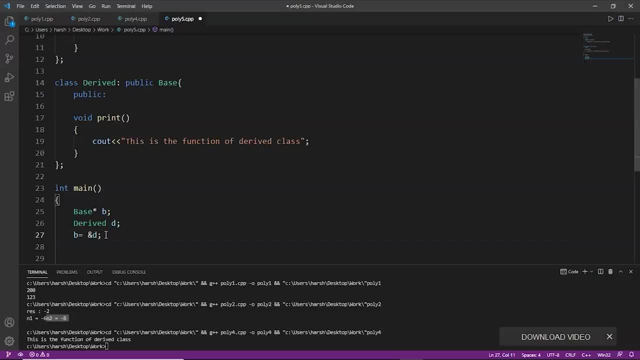 Because The pointer of base class, Which we are using to call the functions, Points to the derived class object. So now Let's do the calling part. All we need to do is The pointer And the arrow operator And the name of the function. 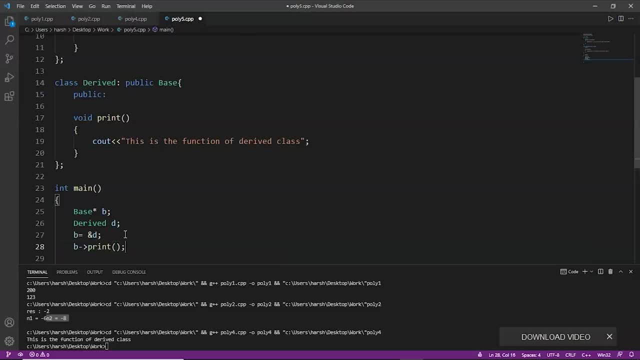 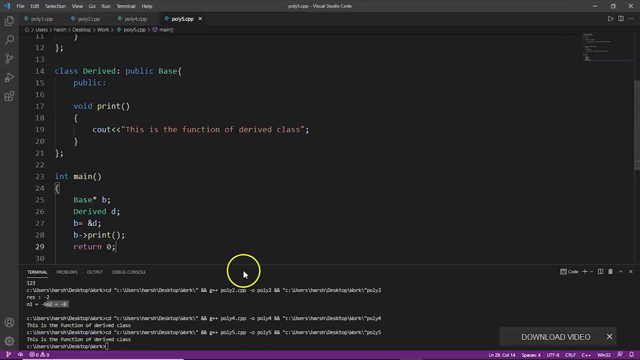 That is, print. After that we can write return 0.. Now Everything is done. Let's save this And run it. As we can see, This is the function of derived class. Here we can see So the derived class function. 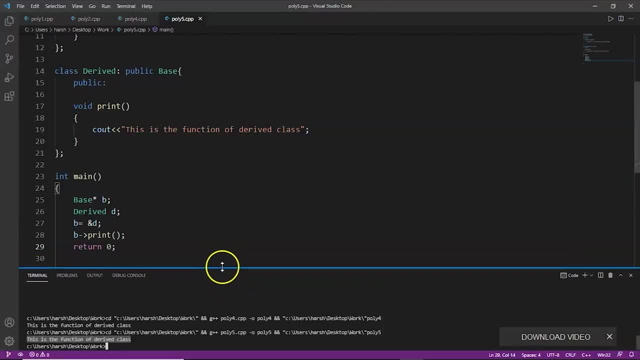 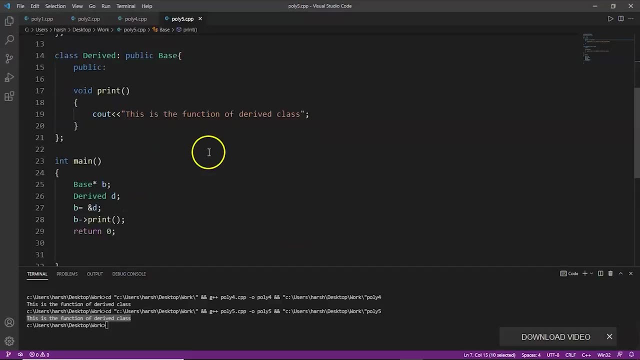 Is getting called, Which we wanted. So this is an example of Virtual function in C++. We have used this virtual keyword over here And, using the Base class pointer, We have called this function. And These were some examples of different topics. 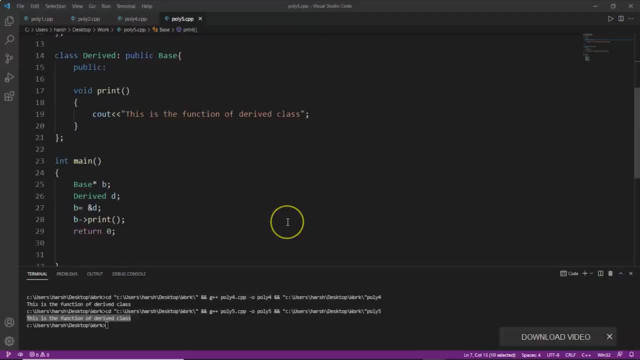 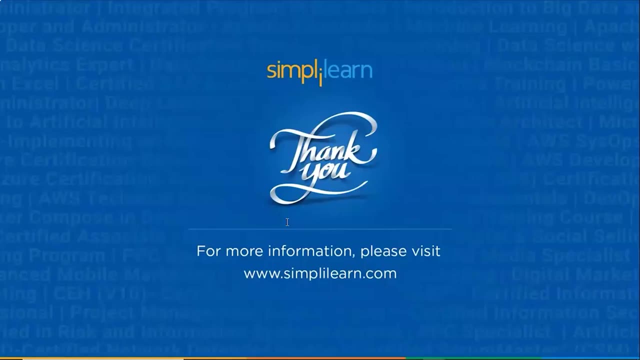 In polymorphism in C++. You can try some more examples On these topics To help you in understanding this topic In a better way. Alright, with that, We have come to the end of this video. If you like this video, Please give it a thumbs up. 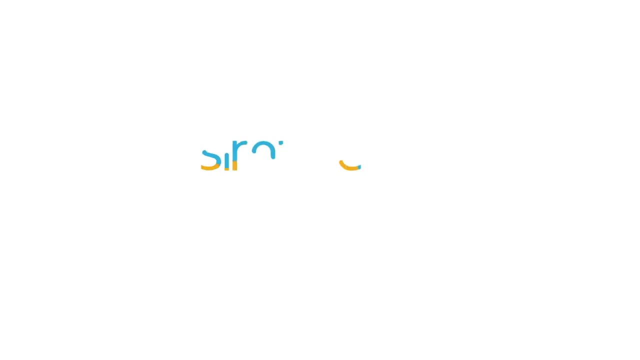 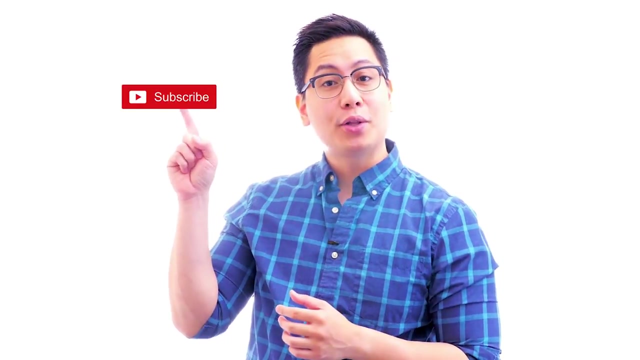 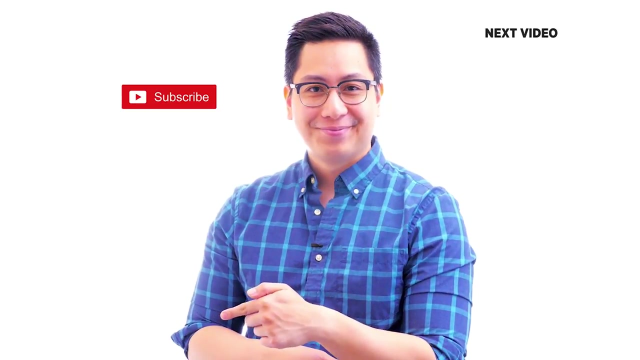 I hope it really helped you all. Thanks for watching, Stay safe and keep learning. Bye. 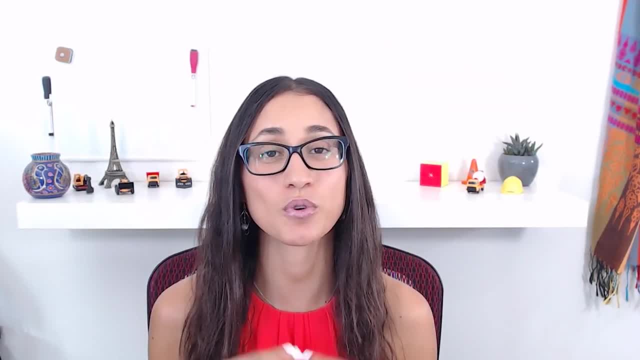 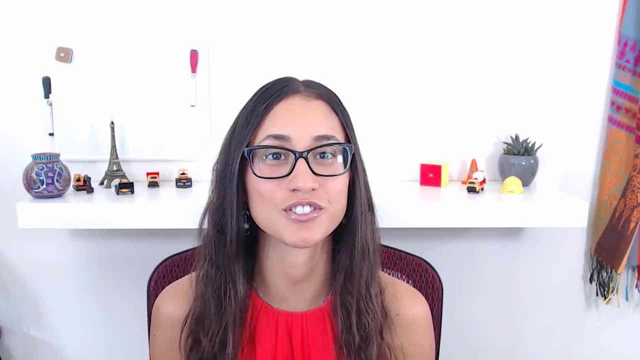 Bonjour, Genie Engineers. In this video we're going to do a lot of practice problems for soil classification. Now, if you're here for the first time and you just want to learn about engineering or just how to engineer like better, don't forget to subscribe and make sure you hit the bell. so 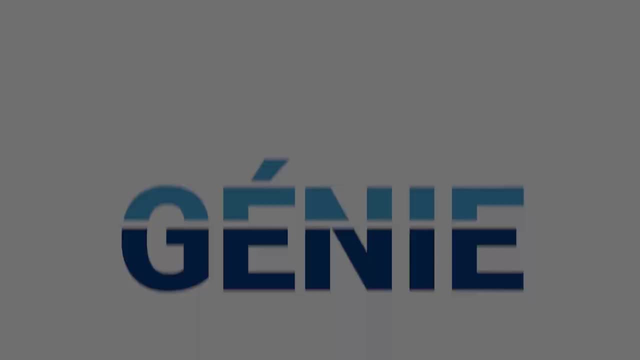 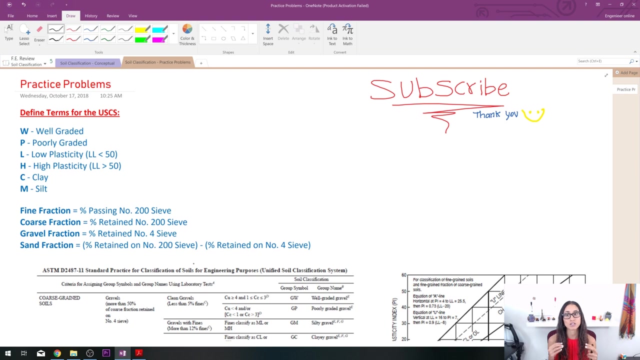 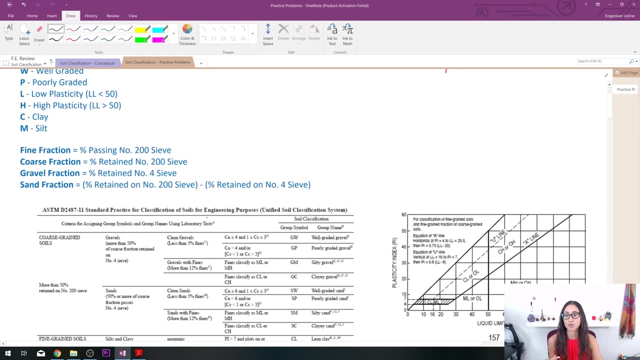 you don't miss out on future videos. Now let's get started. First, I would like to go over some terms that I think it's important to understand before we start solving the problems. Now, if we look at the table USCS, here we have group symbol. It tells you GW, GP. but it's important to just really know. 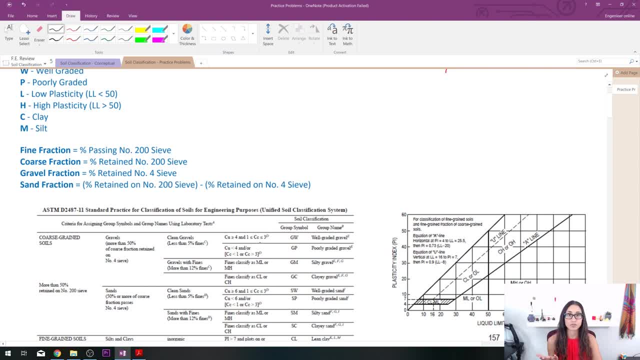 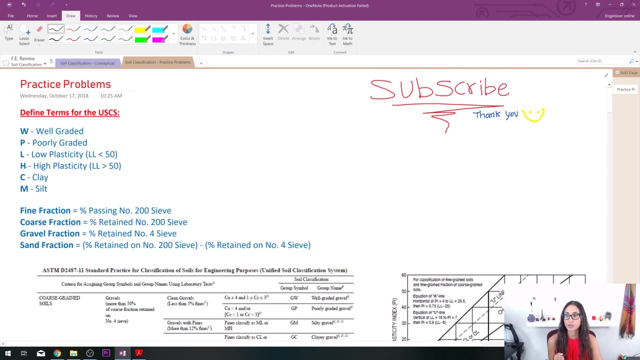 what these stand for. So you have G, which stands for for gravel, S stands for sand. then we have W stands for well graded, P stands for poorly graded, M stands for silt, C stands for clay. then we have what else. we have L: it's low plasticity, and that means liquid limit has to. 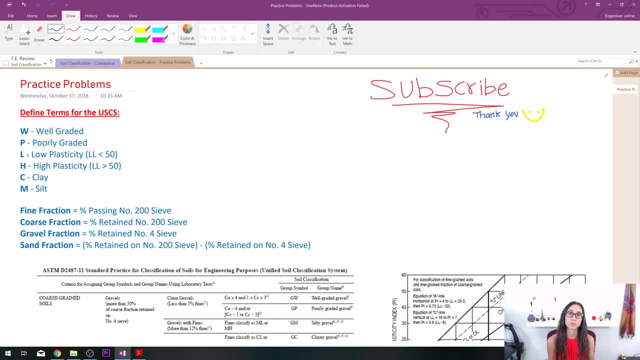 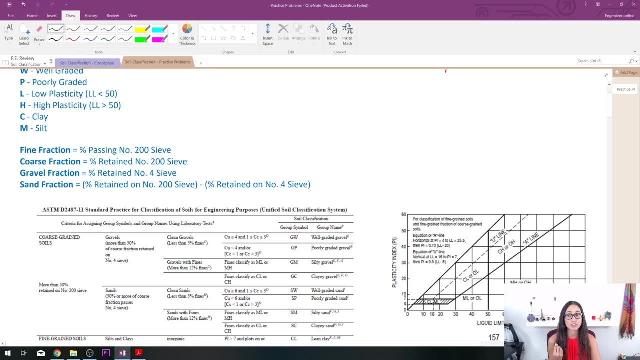 be less than 50, and for high plasticity, your liquid limit has to be greater than 50.. Another term I would like to go over is diffraction. These are really important because a lot of times you found them in the question and so if you don't really understand what it means, it's really hard. 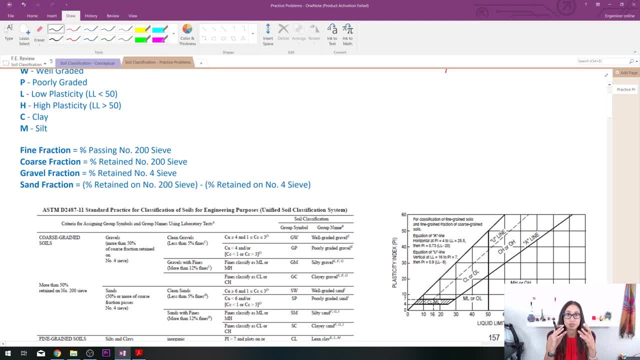 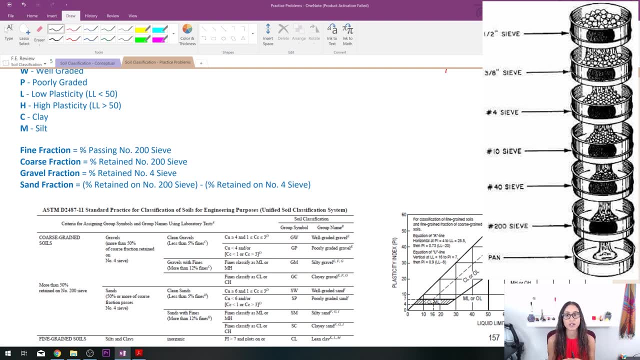 to solve. So we have fine fraction. that just means the percentage that passes a number, see 200.. So if you remember from my previous video when we talked about the sieve analysis, you remember the 200 was the last one before the pan. So whatever passes the 200, that soil.